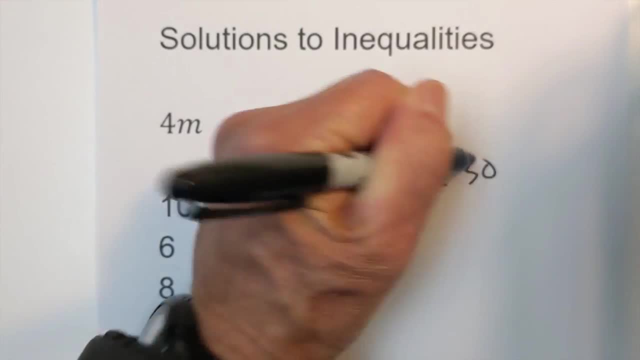 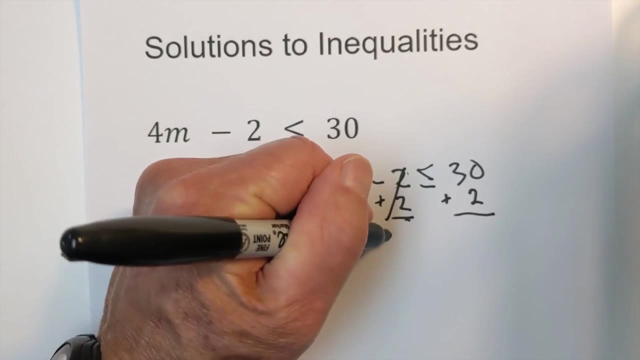 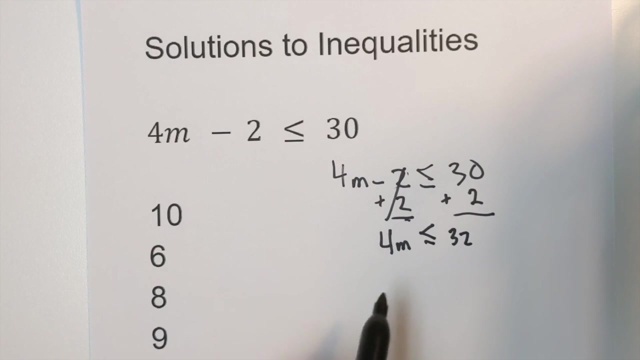 minus 2 is less than or equal to 30. I'll add 2 to both sides. These cancel. I bring down the 4m less than or equal to 32.. Now what I do is I divide by 4 to get the m isolated. 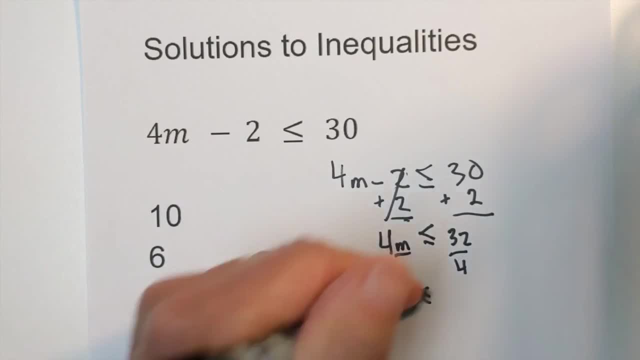 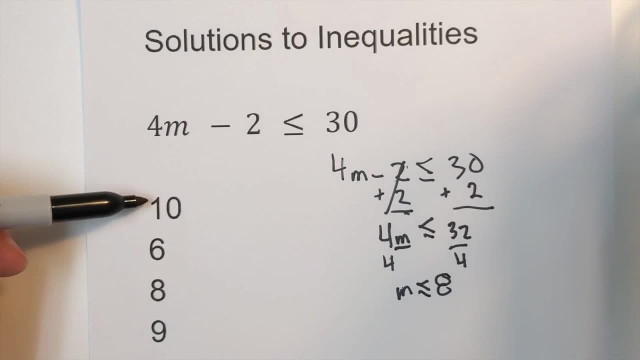 So m is less than or equal to 8.. Okay, Okay, So now that is our solution, Now what we need to do. we have a couple of choices. Which of these satisfy this? less than or equal to 8?? Well, 8 does and 6 does. So our solution: 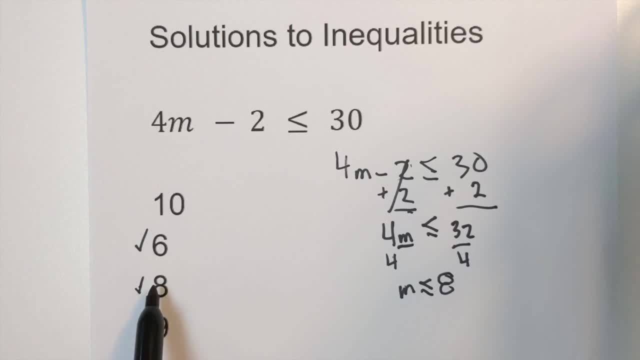 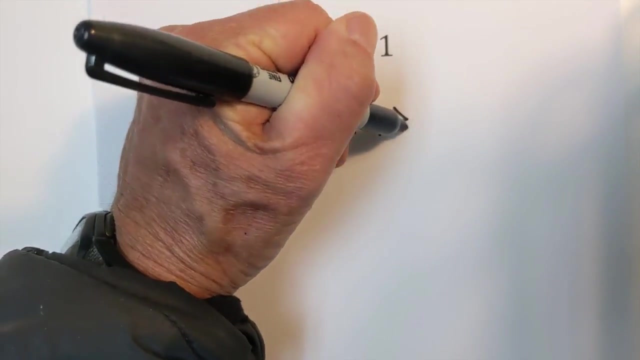 would be 8 and 6, because they're both less than or equal to 8.. Let's work another example. Okay, Again, let's solve the inequality. So I'm going to rewrite: r over 2 plus 4 is greater than or equal to negative 1.. I'm going. 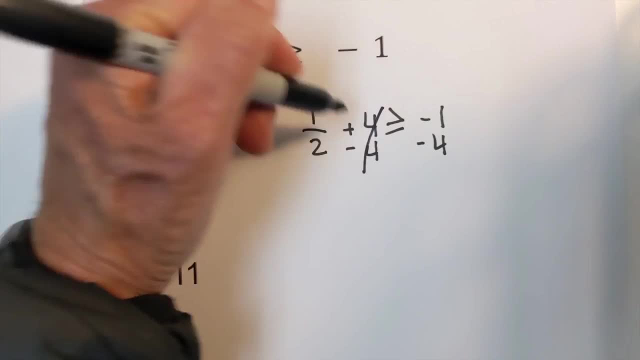 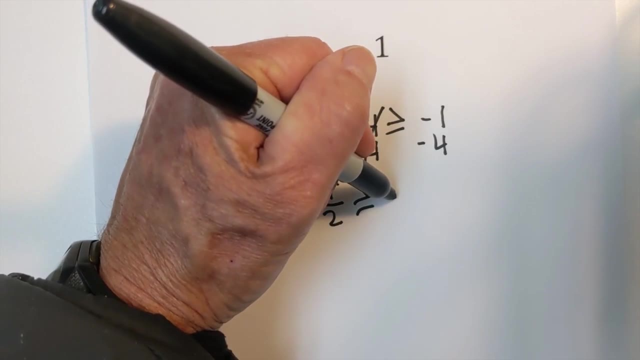 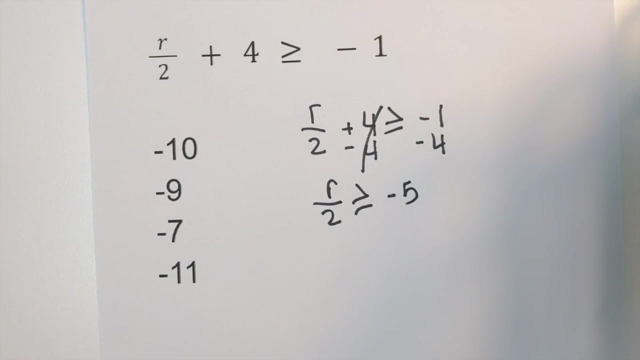 to first subtract 4 from both sides. Okay, These cancel, Bring down r over 2 is greater than or equal to, And whenever you have two negatives, you add them and then keep the sign of negative, So that will be 5.. Now what we do is use the duty to create a norm. Now, 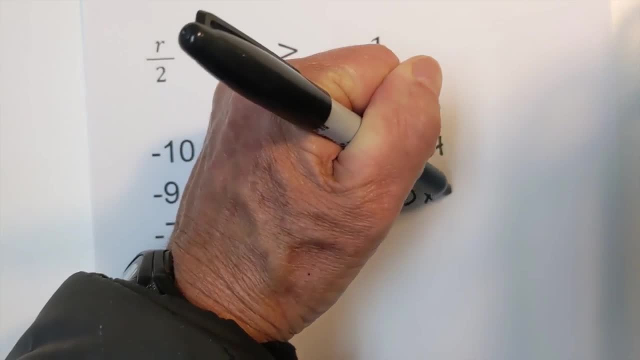 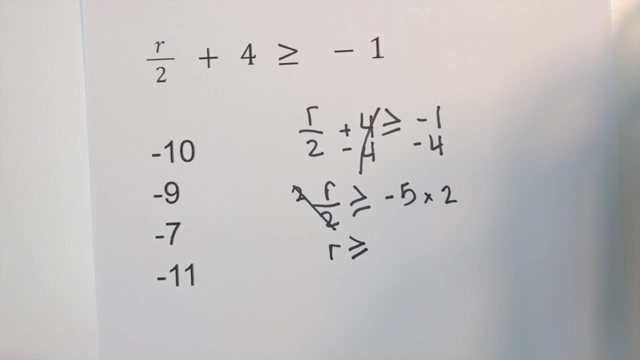 division. so we're going to multiply by 2.. Okay, these cancel r is equal to greater than or equal to a negative times. a positive is a negative, so that will be negative 10.. Now let's see what numbers satisfy this. So it's got to be greater than or equal to negative 10.. So we have negative 10 and negative 11.. 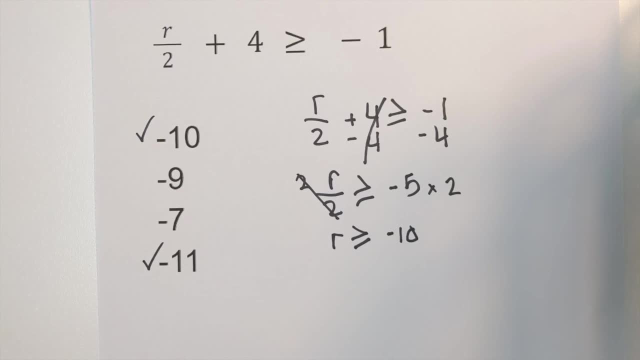 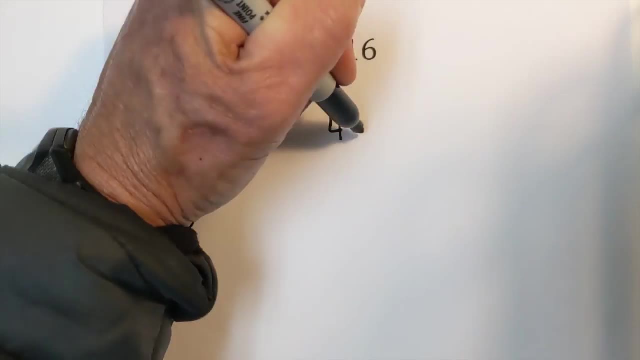 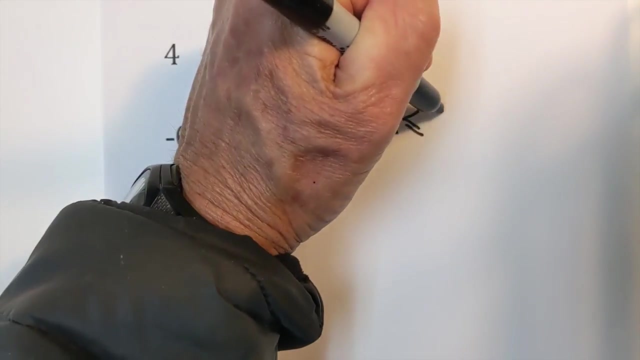 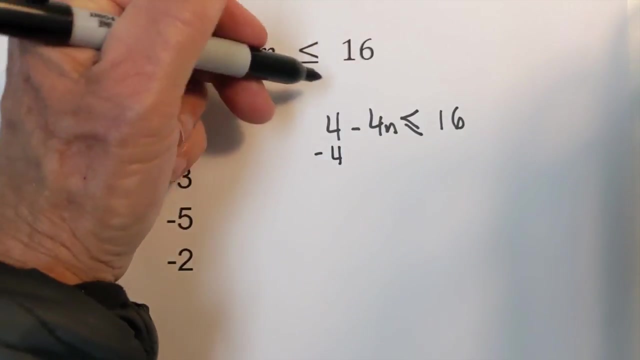 Both of those satisfy this inequality. And let's work. one final example. Okay, let's begin. I probably should have had this written ahead of time, but I didn't. Okay, we have 4 minus 4n is less than or equal to 16.. Let's begin by getting rid of the 4 by subtracting 4 to both sides. Okay, these cancel. You have negative 4n.